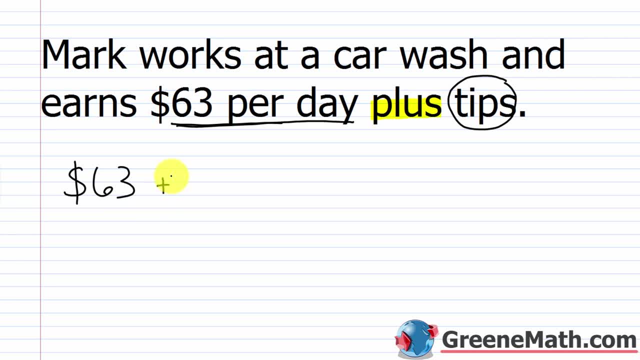 So I'd put $63 plus and let's use the common variable variable of x, so plus x, So this represents the amount, the amount of tips. Now we can use this to model what this person, Mark, is going to receive every day. He gets $63 plus x, where x equals the. 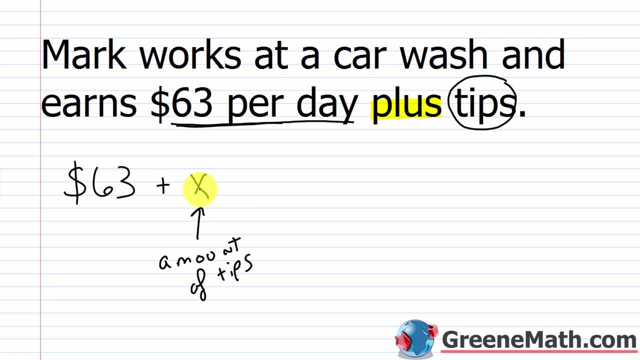 amount of tips that he's going to receive. So let's say the day is over and he knows that he got $63 plus x. He's going to send me an extra $7 in tips. So x in this case would equal 7.. If I want to, 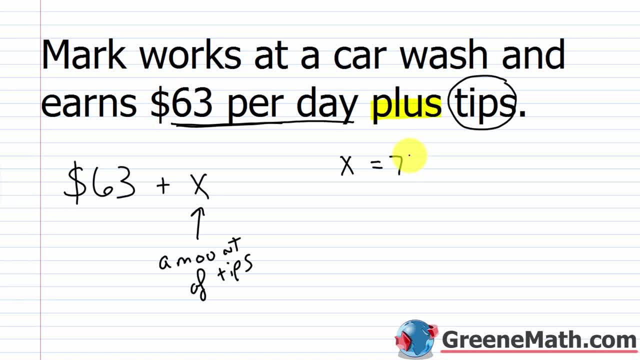 know how much he made for that day. all I would do is I would take this right here, this 7, and I would plug it into the x right here, because x equals 7.. He got $7 in tips. x was the amount of. 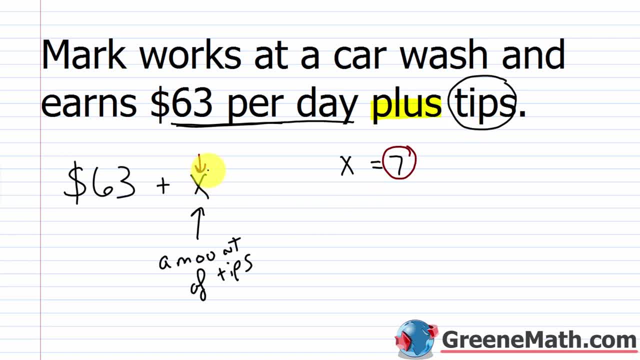 unknown tips he was going to get, And so we plug in a 7 for x and we'd end up with $63 plus 7. And put dollars there, just to be consistent, And this will equal $70, right, That's how much he received. 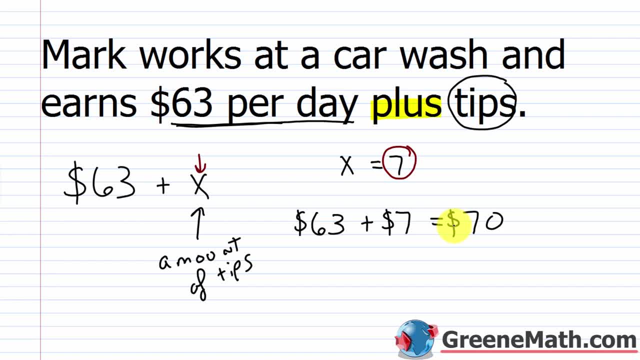 for that day, But the next day it's going to be different. So let's say, the next day X is going to equal nine. Well then I take 63 and I'd add nine to that. right, I'd make two more dollars. 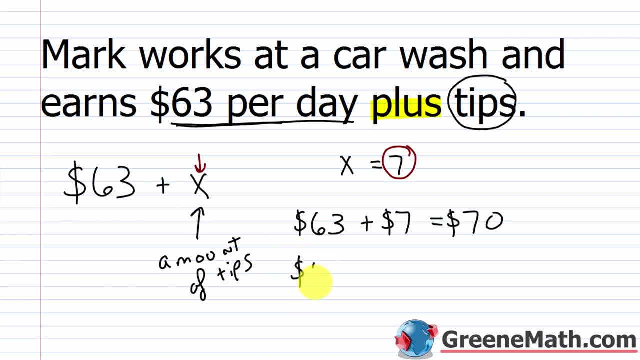 or I'd have 72.. So the following day you would have $63 plus. and let me do this in a different color so we don't get confused. $9, right? So in that case X is equal to nine. So we see that. 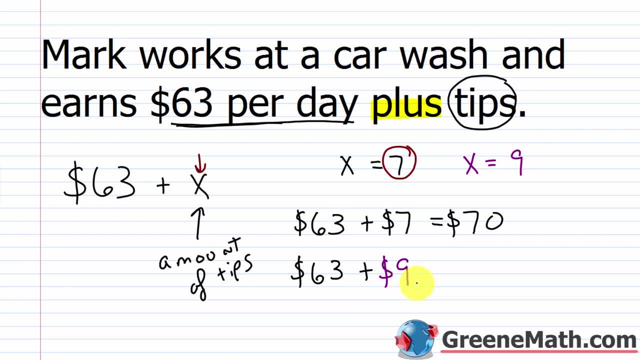 as we change the value for X, the value is going to change. In this case, X is equal to seven. I plug in a seven for X and I get 70, right, 63 plus seven is 70. And the other case, X equals. 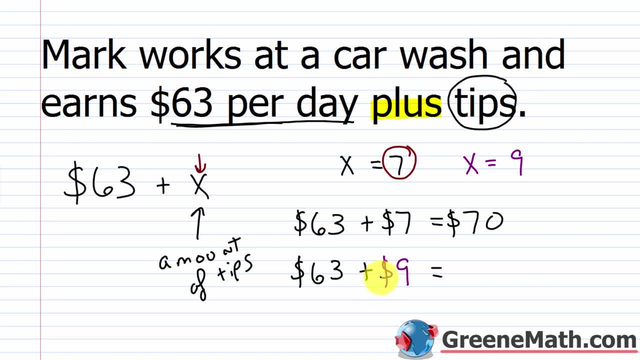 nine. So I plug a nine in for X. 63 plus nine is going to give me 72. So he earns $72 in this case. So I plug a nine in for X 63 plus nine is going to give me 72.. So he earns $72 in this case. 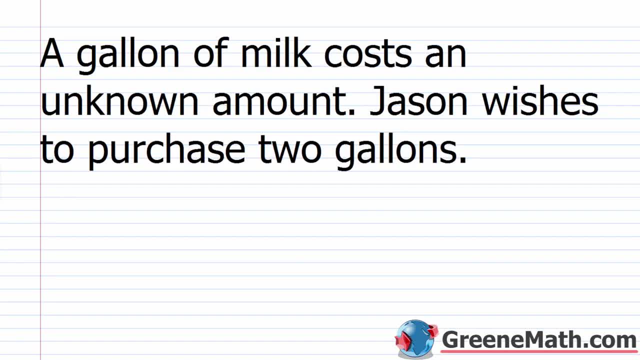 Let's take a look at another one in case you're a little confused. So a gallon of milk costs an unknown amount. Jason wishes to purchase two gallons. Well, again, we can use a variable to model this situation. So I know that he's going to buy two gallons. So that's two, And 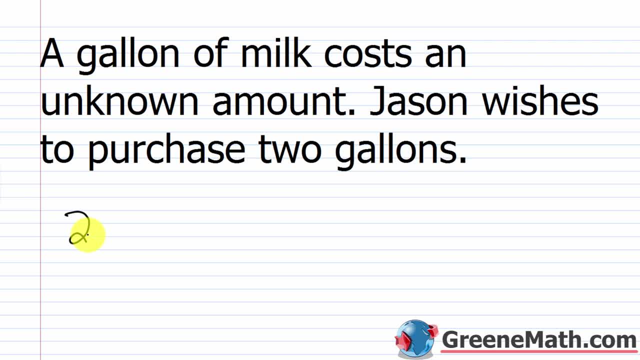 it costs an unknown amount. So I can use a variable. Let's use Y in this scenario to represent that. So I need to multiply the cost per gallon times the number of gallons. The number of gallons is two. The cost per gallon is unknown, So I would have two times Y. 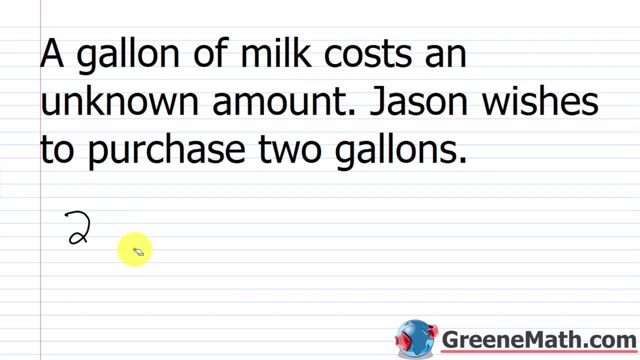 which we're going to write as just two Y. Okay, when a number is next to a variable, it implies multiplication. So two Y like that is telling me that I have two times Y or two times Y. You remember back in pre-algebra when I said: we stop using this symbol to imply: 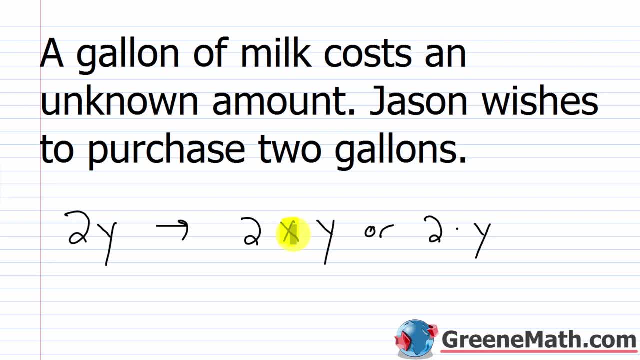 multiplication, And the reason is is because it often gets confused with the variable X. So we'll either use this symbol, or we'll use parentheses, or we'll place the number next to the variable, And this is the most common. You'll just have two times Y, like this: 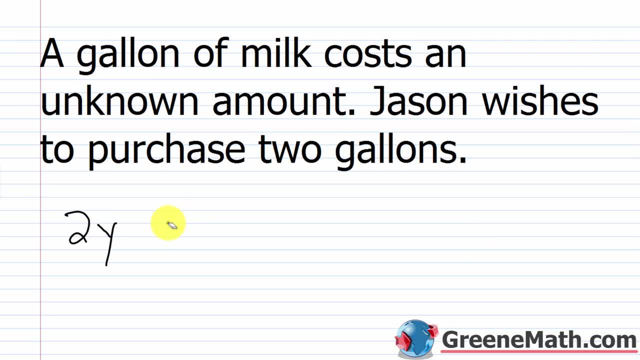 just two Y. That implies multiplication. Now if I give you a cost per gallon of milk, I can tell you how much Jason's going to spend on his milk purchase. If I say that Y is equal to $1, and I'm not going to put the dollar symbol in this time, I'm just going to put one. Well, 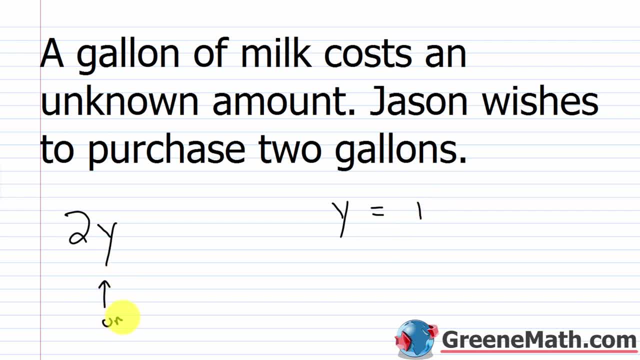 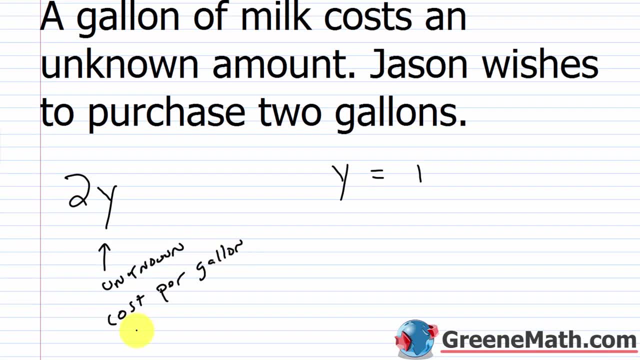 then really all I'm going to do is plug a one in for Y right. This is the unknown cost per gallon of milk. If I tell you that it equals $1, I could just plug a one in there and I could say okay. 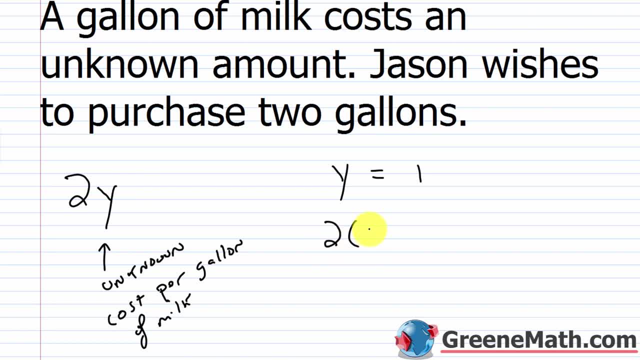 well, two times one is two, So two times one is two, So he spends $2 on two gallons of milk. If that amount changes, right, if it changes, if I say: well, the price of milk just went up, So 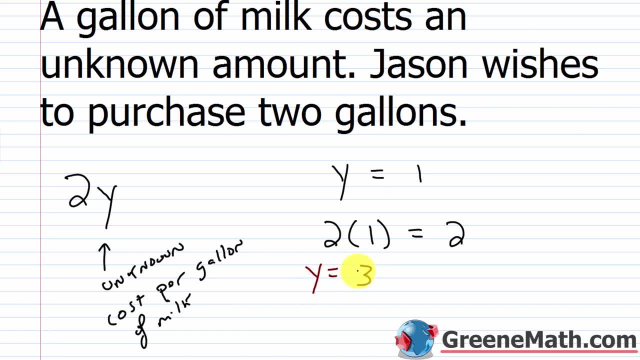 let's say that now Y is going to be equal to three. Okay, we had a big price increase. Well, now I'm going to plug in a three for Y. So instead of two times one, I would have two times three. 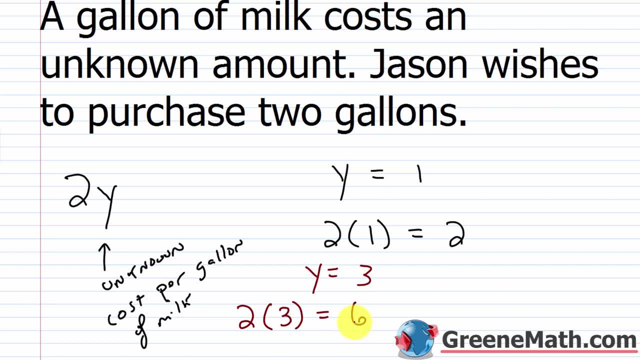 and that's going to give me six. So now he's going to spend $6 on two gallons of milk. right, And that makes sense. Two times three is six. So if Jason's going to spend $2 on two gallons of milk, 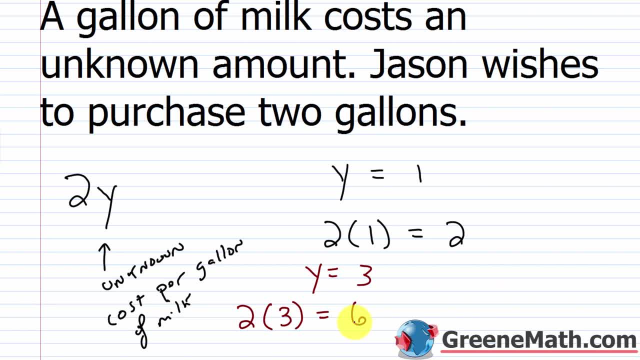 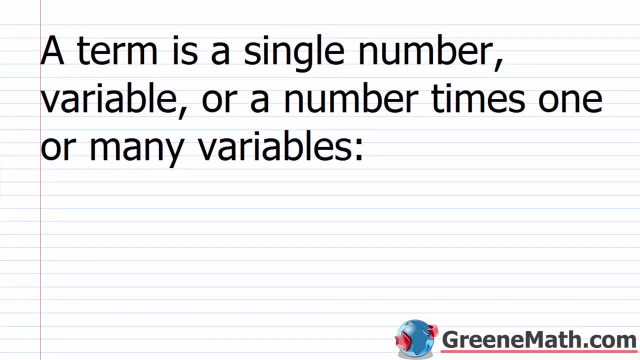 Jason buys two gallons of milk at $3 per gallon, he spends $6.. And the other scenario: if he buys two gallons of milk at $1 a gallon, he's going to spend $2.. All right, so let's get into some more. 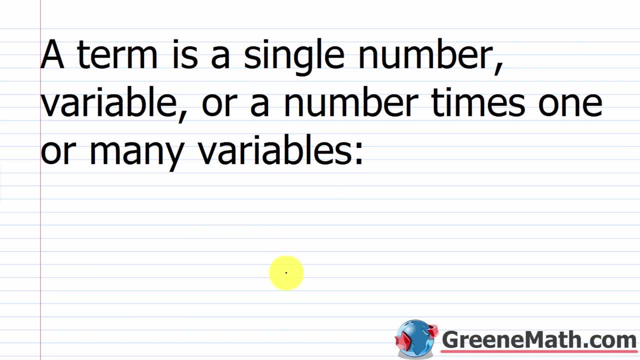 kind of definitions. A term is a single number variable or a number times one or many variables. So, for example, you might see something like 4X- Hey, that's a term. Or you might see something like 9Y. 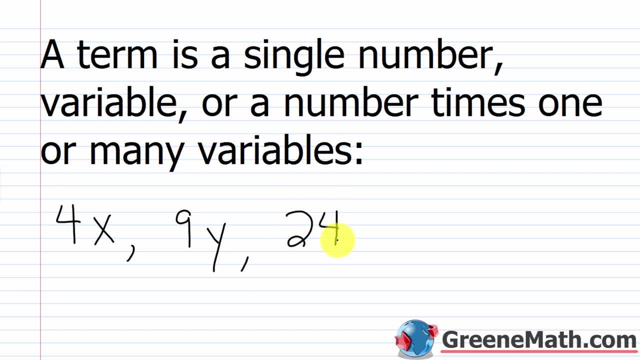 That's a term, Or you might see something like 24XYZ, Or you might see something like negative 3A. These are all examples of a term, right, A single term. Again, it's a number by itself. So if I just had, let's say, the number seven, that's a term, Or it's a number times one or many. 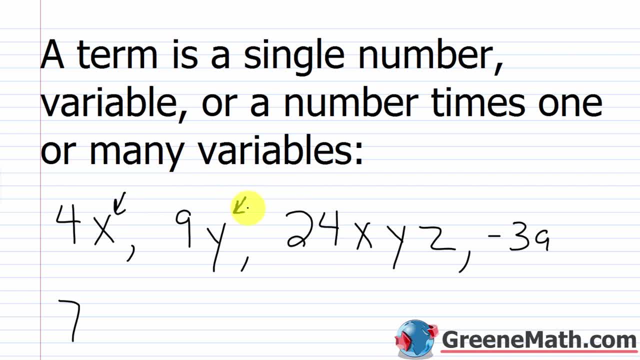 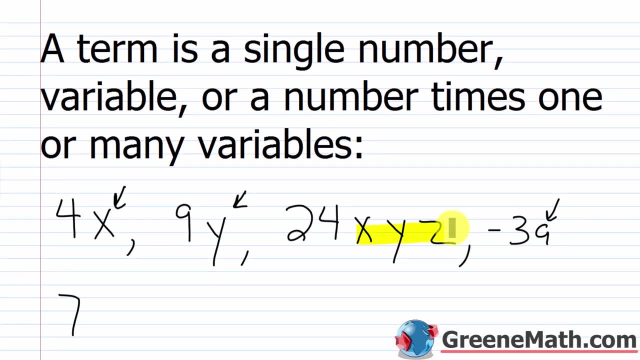 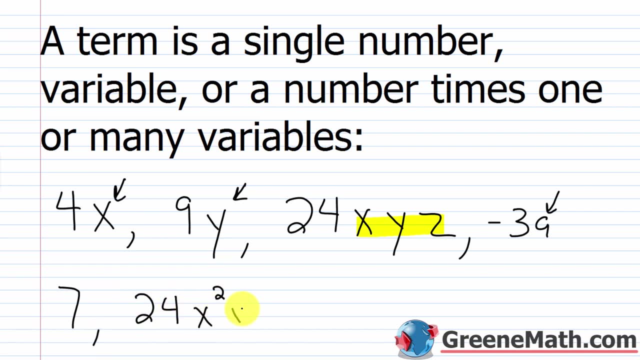 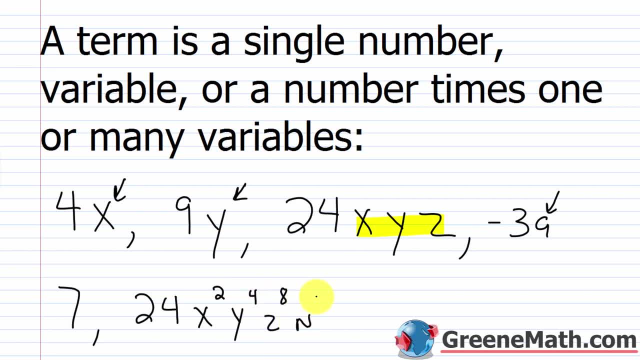 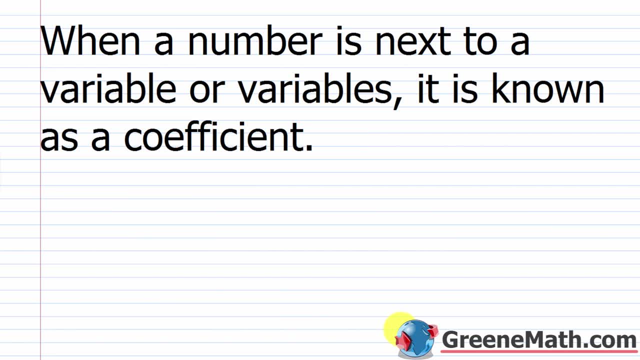 the fourth, Z to the eighth, let's say N to the 12th. That's a term right, A single term. Now here's another kind of definition thing: When a number is next to a variable or variables, it is known as a coefficient. 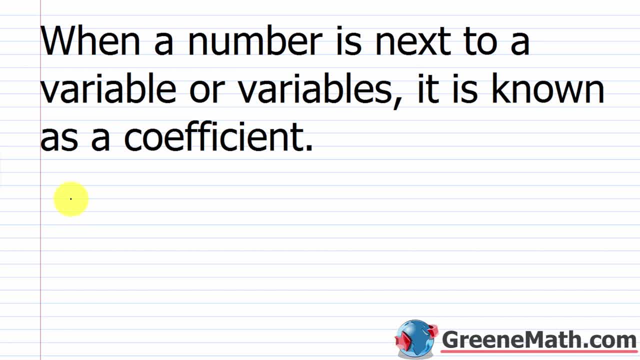 So in all these scenarios where I'm saying, okay, two times Y, right, Two Y is how we would say it, but two times Y really, because it's multiplying. Two is the number that's multiplying the variable Y. It's known as a coefficient. Two is the coefficient of Y. If I had, let's say, 4X, 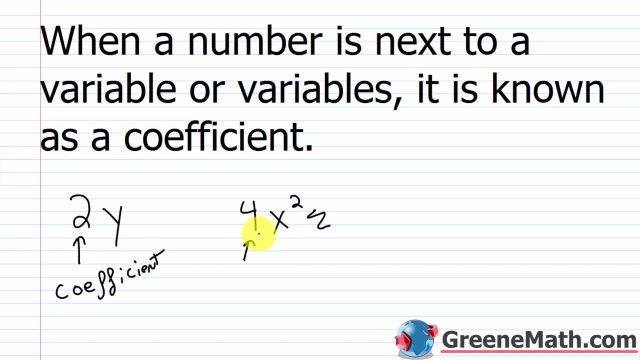 Z four is the coefficient right It's the number that's multiplying the variable, or again variables if you have more than one. So this is again a coefficient And these are kind of very basic definitions that, even if you don't get them in this video, 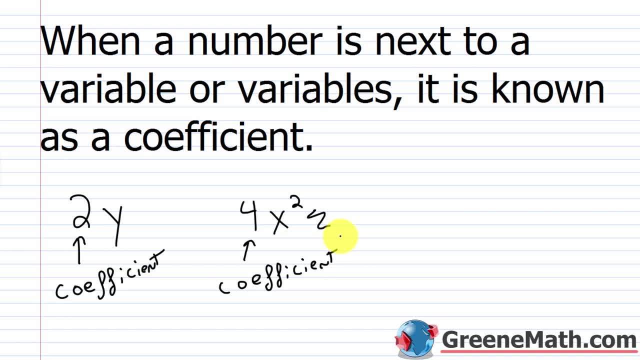 you can write them down and put them on flashcards if you want. We're going to talk about them over and over and over again. By the time you get to the 10th lesson, you will know all of these terms right. It won't be an issue for you. 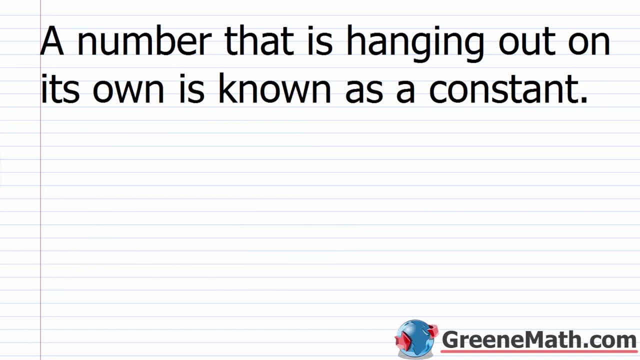 All right. So a number that is hanging out on its own is known as a constant. So you're going to get to a point in this lesson where we start talking about algebraic expressions and you might see something that looks like 5X plus seven. So this number, this seven, that's. 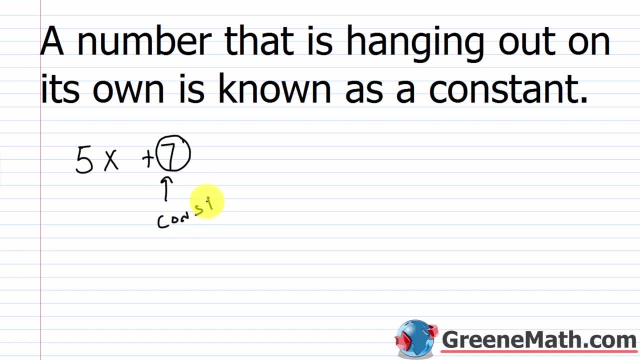 hanging out by itself is a constant. This is a constant. Its value is not going to change. It's what we've worked with in pre-algebra. right, Where we're just doing basic operations. If I do seven times three, that value is always going to be 21,. right, It's not going to change. 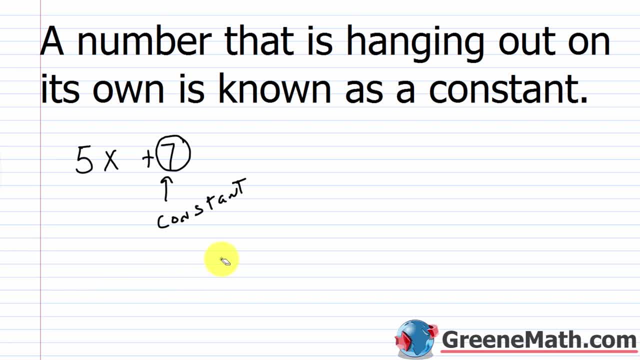 because we're working with constants. If I have five X plus seven, well, I don't know what the value of X is. Again, it's allowed to vary, It's allowed to change, And so the value for this is going to change based on what X is. If I change X, I change the value of this whole algebraic. 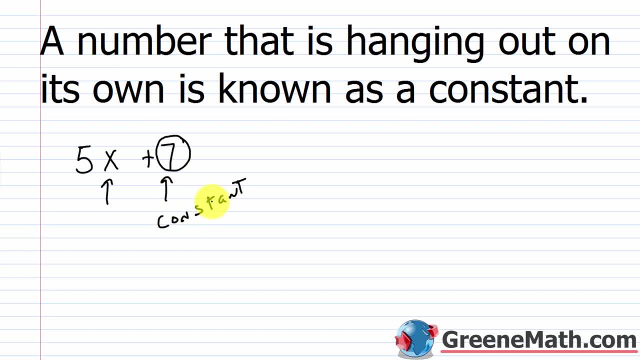 expression. So that's kind of the difference here. That's why we say this is a constant, Because the number seven is not going to change. If I have something like three X squared minus two, two is hanging out by itself. Two's value is constant, It's not going to change. 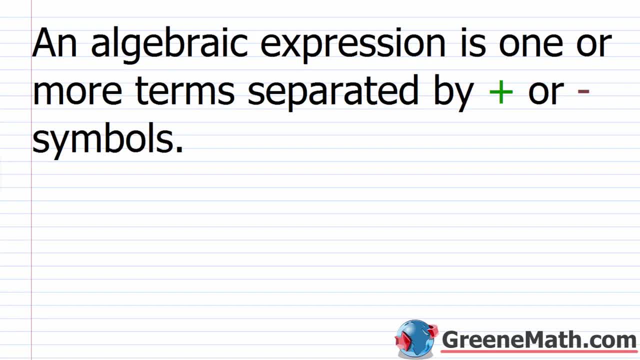 So that's why we refer to it again as a constant. All right, So here's a pretty important definition. An algebraic expression is one or more terms separated by plus or minus symbols. So, again, your terms in an algebraic expression are separated by the plus and minus. 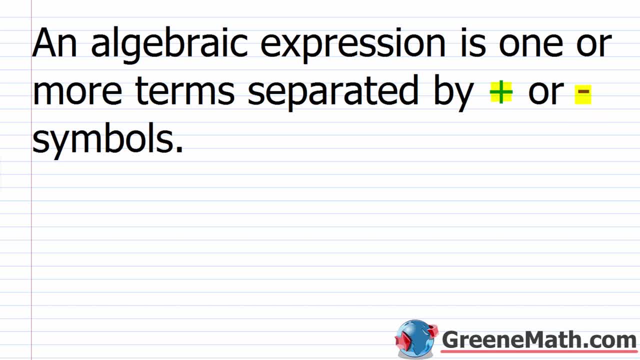 symbols, symbols very important. so let's look at an example. let's say we have something like 5x plus 2y minus 4z. so if you want to look at that algebraic expression and say where are the individual terms, well, every time you see a plus or minus sign, you've cut off a term. so this is a. 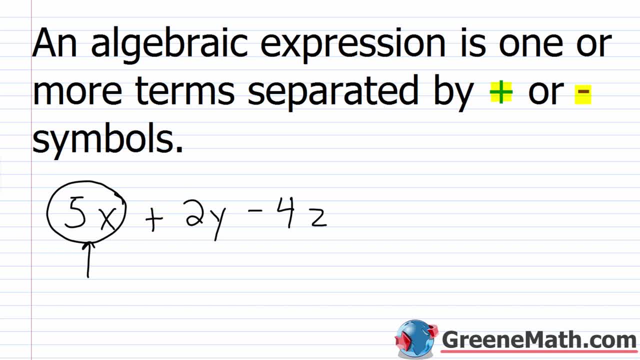 term, this 5x, because there's a plus here, right, that cuts off this term from this term. then this 2y is a term, right? you have a minus sign here and you have a plus sign over here, so it kind of it kind of separates everything. let me just kind of draw a line here in a different color. this: 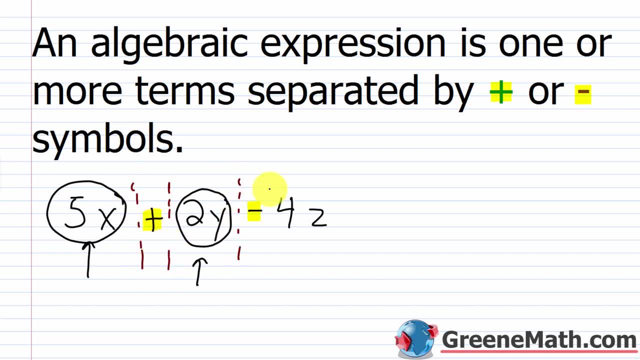 kind of separates everything. and then here where you have 4z, again that's a term, so you have 5x, 2y and 4z. that make up the terms here And it's called an algebraic expression because there are variables involved. If we just kind of have numbers involved, we just refer to that as an expression. 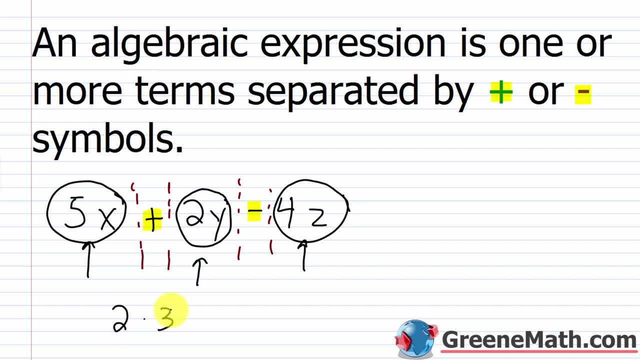 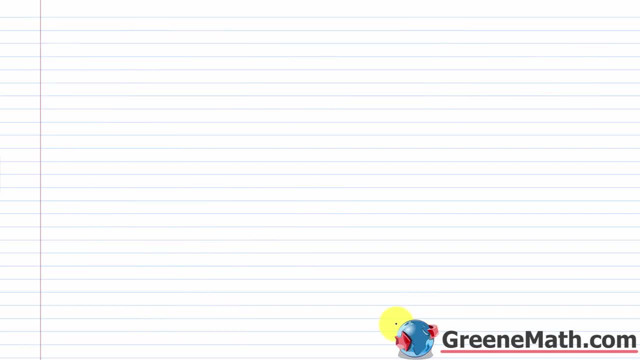 right. So if you had something like you know, two times three, that's an expression, right? We work with that in pre-algebra. So two times three is six, All right. so the main thing about an algebraic expression is that the value will change as its value given for the variables involved. 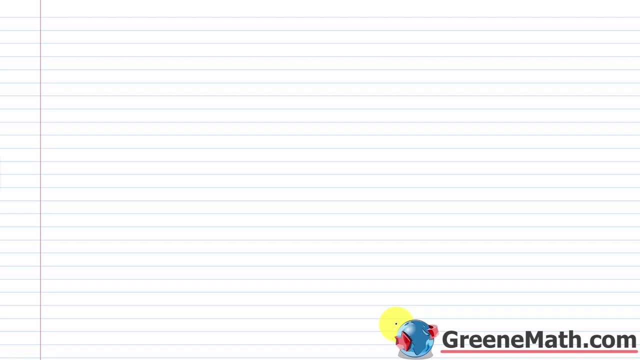 are changed. So let me give you some examples. Let's say we had something simple like 2x plus three And I say I want to let x. let x equal four. Well, what I'm going to do is, everywhere I see an x in the algebraic expression, I'm going to plug in a four. So I'm going to take this value. 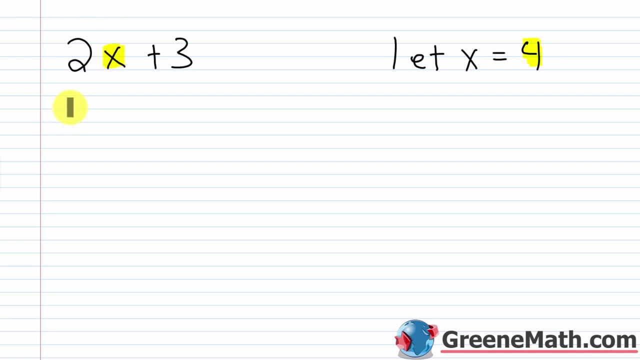 and plug it in here. everywhere I see an x, So that means that I'm going to plug in a four. I'm going to have two times four plus three, And again I can put parentheses around four and put it next to two and it implies multiplication. Remember 2x is the same as two. 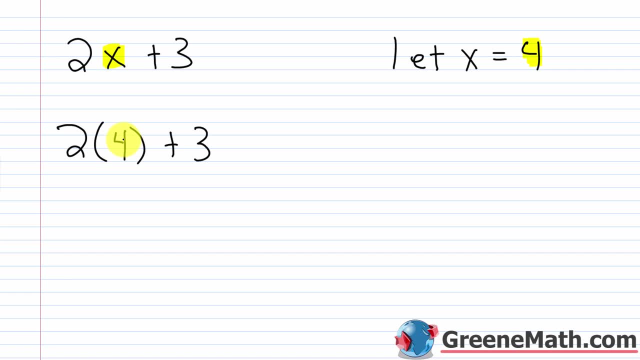 times x. So when I replace x with four, I'm still going to do the multiplication operation. But now, since it's not a variable, it's a number that I replaced the variable with, I can just calculate right: Two times four is eight, So this would be eight. 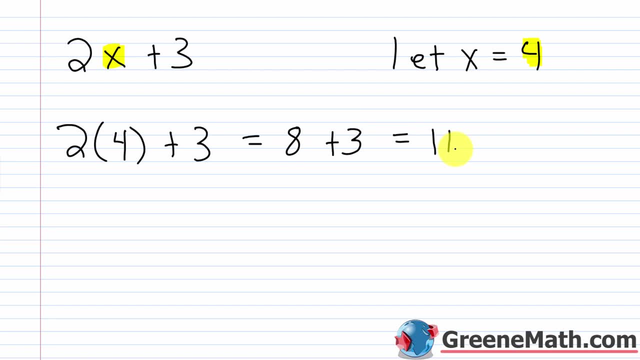 times four plus three, And again I can put parentheses around four and put it next to two plus three, And then eight plus three is 11.. And again I did the multiplication first because of the. please excuse my dear Aunt, Sally right, Remember your order of operations. This is where 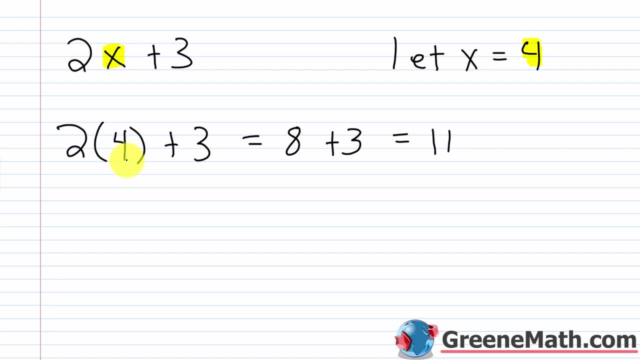 you're really going to use them. All right. So let's say we change the value of x. Let's say, let's say we want to let x now equal, I don't know. let's say five. So instead of plugging in a four for x now, I'm going to say, well, two times five plus. 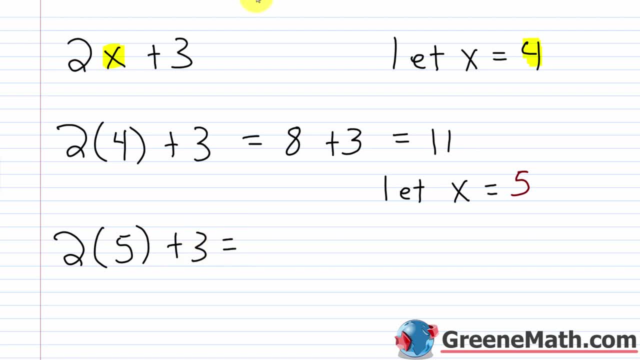 three is going to equal what? Again, I'm plugging in for x, whatever value I let x equal. So that's why there's a five there. And so we just calculate: two times five is 10, then 10 plus three is 13.. 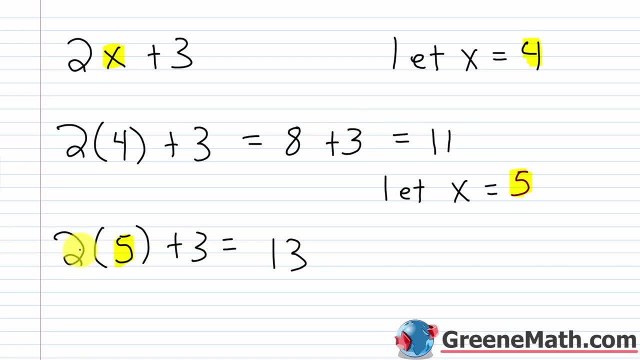 Right, And I did that one step versus two up here. Hopefully you can follow right. Two times five is 10, then 10 plus three again is 13.. So as I change the value of x, the value of the algebraic, 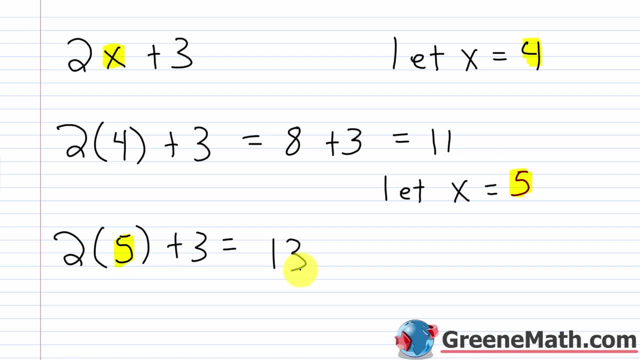 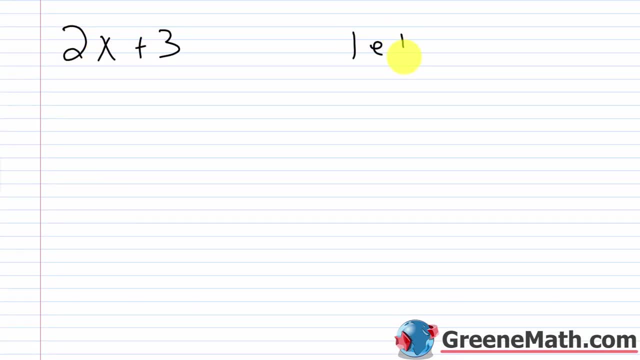 expression will change. Let's do one more. So let's say: well, two times five is 10, then 10 plus more. Let's say again: two x plus three. Let's let x equal negative two. So I'm going to plug in. 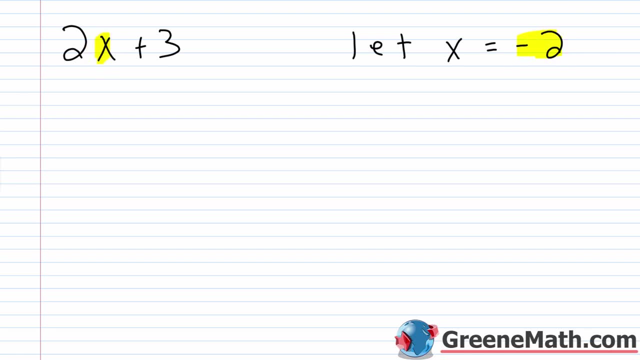 a negative, two for x, right. Very, very simple. So two times negative two plus three equals what: Two times negative two- Remember positive times negative is negative. Two times two is four. So that's going to give me negative four then plus three. 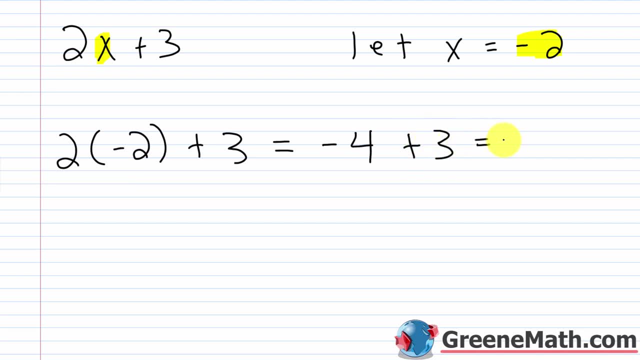 And at this point we know how to add integers right: Negative four plus three is negative one, All right. So again, in each case we got a different value for the algebraic expression because we chose a different value for our variable x. So in some cases we can simplify. 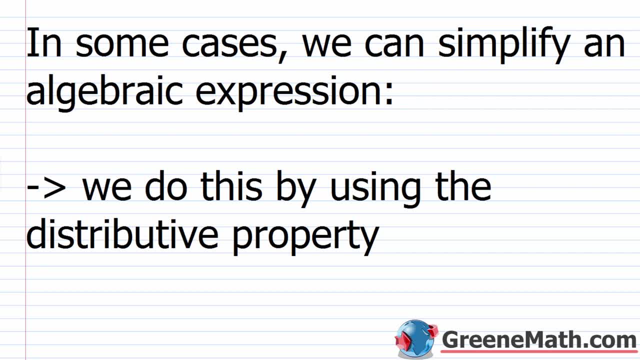 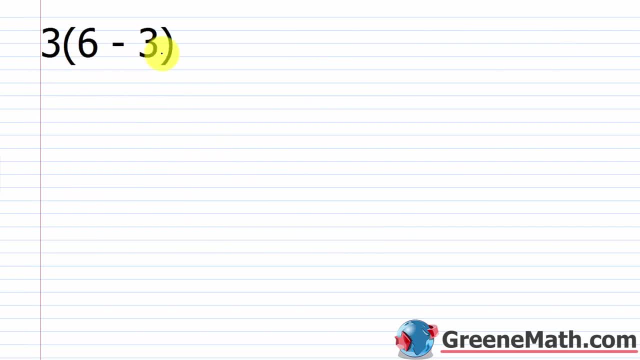 an algebraic expression And we're going to do this using the distributive property. So we learned this back in pre-algebra And to give you an idea of what the distributive property is, we're going to use the distributive property. And to give you a basic reminder of this, let's say we had something like three times. 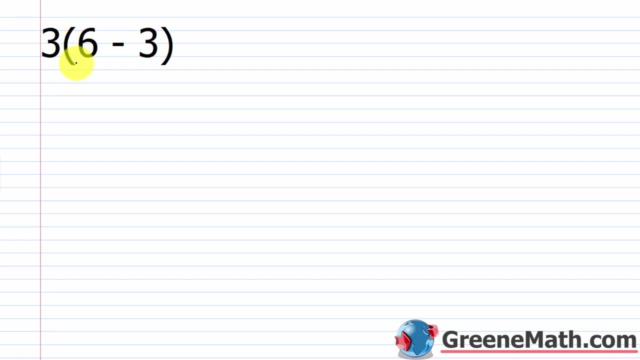 this quantity six minus three, Again, because we have parentheses here. I'm basically saying: what is three times the difference of six and three, right? So six minus three is what That's three. So three times three is nine. But we can use the distributive property to do this as well. 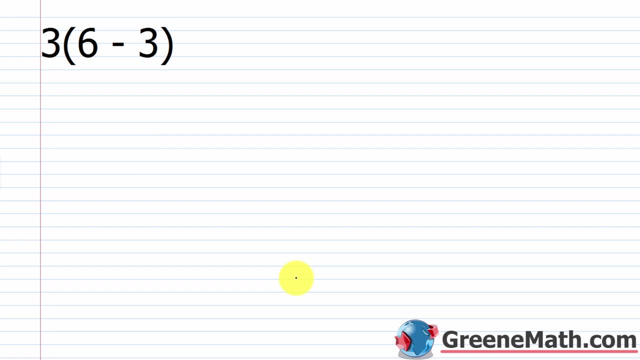 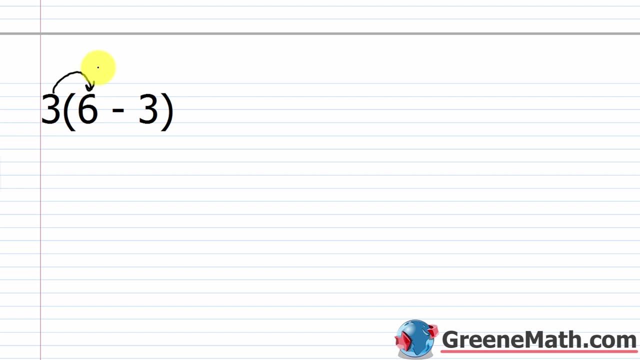 Remember, because multiplication is distributive over addition or subtraction. So what I can do is I can distribute the three to each term, inside of the parentheses. Remember, if I have a single number, that's a term, right, A single number that's a term. So three times six. 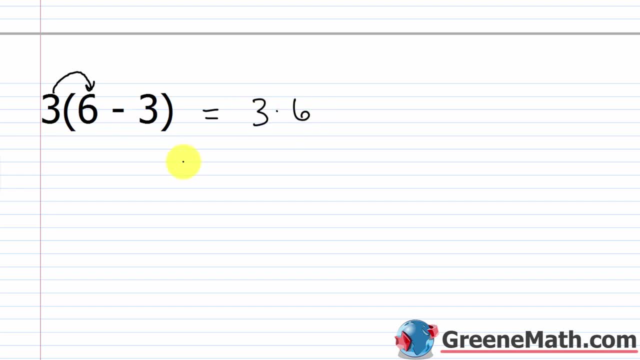 would give me 18.. But let's write it out like this: And then, minus, you'd have three times three. three times three, I'll get the same answer as I did before. right, I'm going to get nine either way. Three times six is 18.. And we're going to use the distributive property to do this as well. 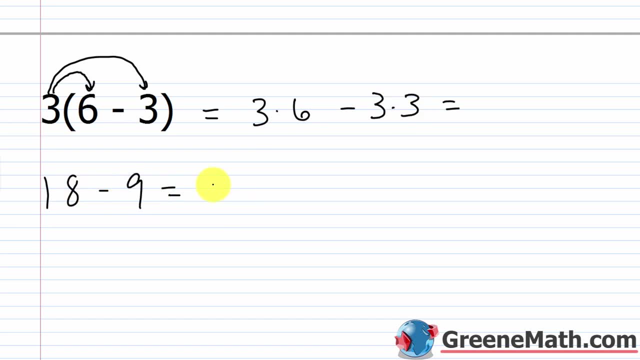 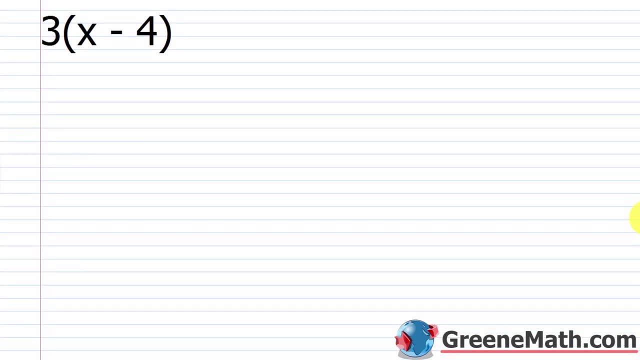 We're subtracting away three times three, which is nine, And 18 minus nine is nine, right? So either way you do it, you get the same answer. So we're going to use that property here to simplify. We have three times this quantity, x minus four. So what I'm going to do is I'm going to distribute. 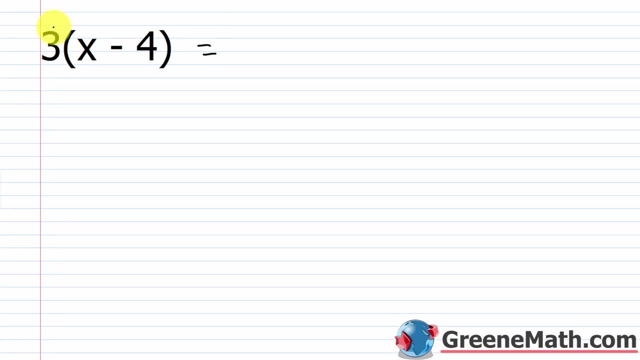 this three to each term, inside of the parentheses. So three times x is three x then minus three times four, which I can write three times four, I can just say 12, right, We know that's 12 at this time. So I've simplified three times this quantity, x minus four, as three x minus 12.. Now I don't have 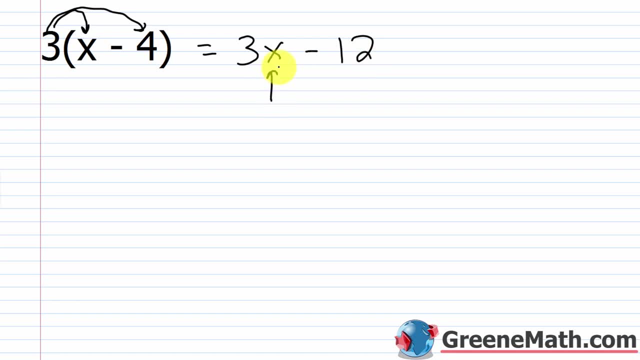 a single number here as an answer, because I still don't know what the value of x is. But I've simplified it a little bit, or some people in some cases are going to want to write it this way, And we'll learn about that later on in algebra one, where we're going to reverse what we just did. 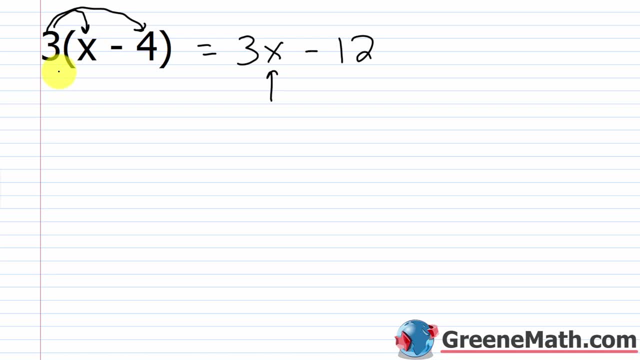 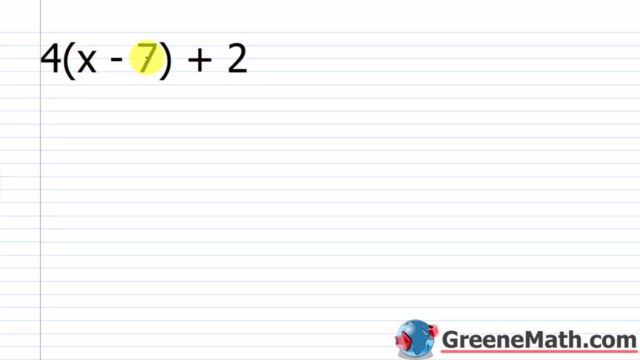 That's a process called factoring, And again, we're not going to talk about that now. That'll be in a much further lesson. All right, let's take a look at another one. We have four times the quantity x minus seven, plus two. So what I'm going to do is I'm going to multiply four times x, I'm going to distribute, So that'll be four x, And then we'll have four times seven, that's 28.. And then plus two. So at this point I don't know what four x is right- I don't have a value of x- But I do know what negative 28 plus two is right. I can do that. And again, if I have minus 28,, 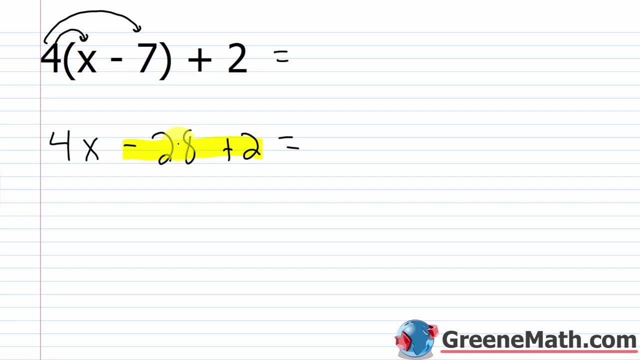 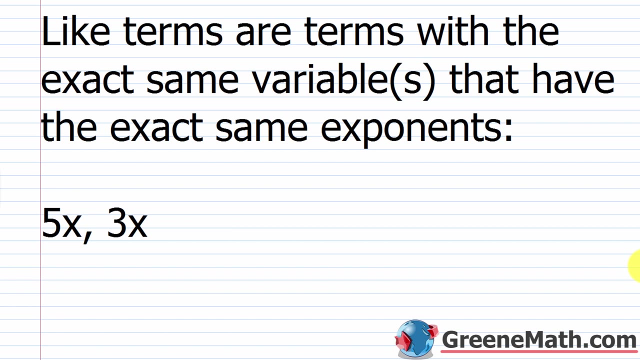 that's the same thing as plus negative 28.. So that's why I said it that way. So negative 28 plus two is going to give me negative 26.. So we would have four x minus 26.. All right, now let's talk about like terms. So like terms are terms with the exact same variable, or variables. if there's more than one that have the exact same exponents, All the variable parts have to be the same. I can't stress that out. 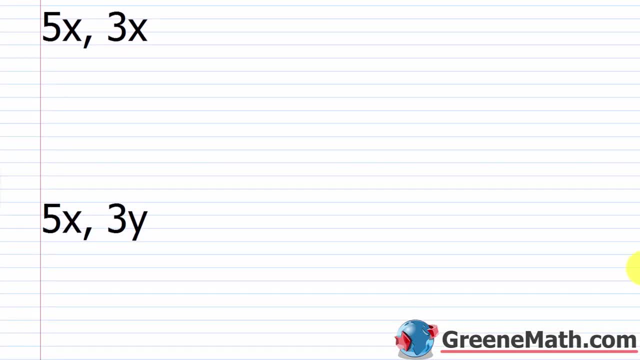 that enough. so, for example, 5x and 3x are like terms are like terms. it does not matter what the coefficients are, right, remember, that's the number, that's multiplying the variable, or again, variables. it only matters what the variable or variables are. in this case, we have X. in this case, we have X, it's. 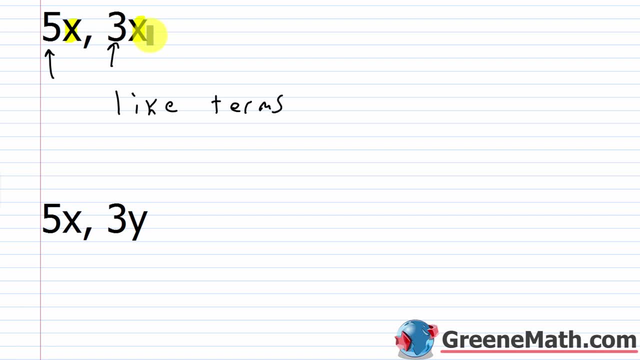 the exact same variable, and so we have like terms. let's look at 5x and 3y. I have X and then I have Y. those are not the same, not the same right? they're different letters, so they're not the same, and so we do not have like terms. 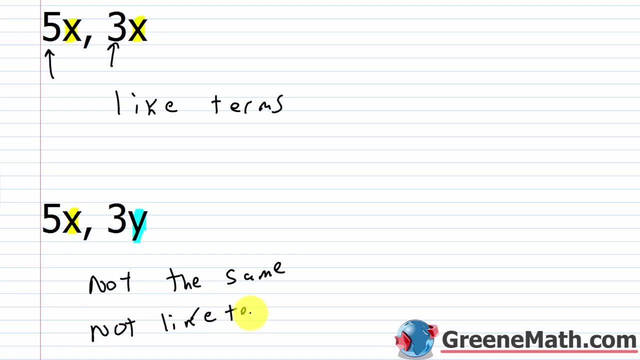 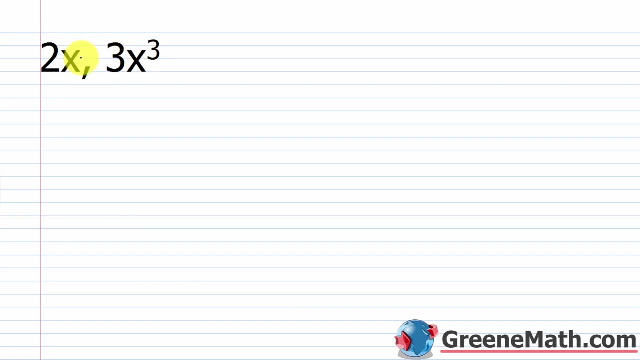 these are not like terms. what about 2x and then 3x cubed? well, they both have the variables that are like terms, and so we have like terms, and so we do not have 5x and then we have Y. those are not the same, but they're not equal. we have the. 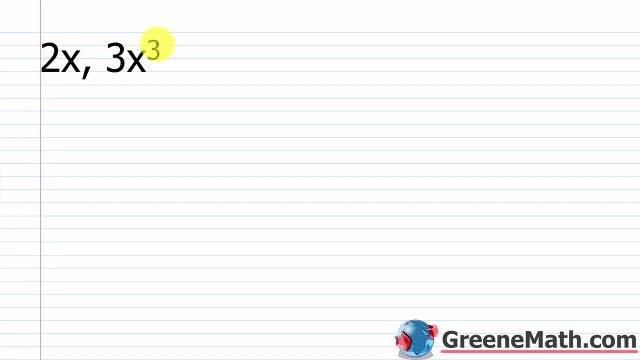 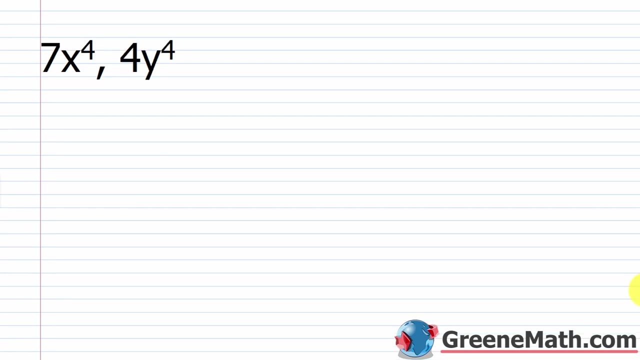 variables which are also увеличed. we have the same순al variables, the variables which are also увеличed. we have 2y squared, but they're not like terms, right? so that's gotta be significant of this letter, that's gotta explain why. so what does that do here? well, you do so. you have an. 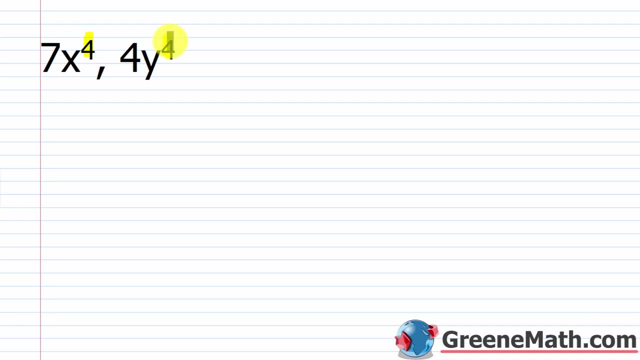 variable itself is different. One is x, one is y. You can't have anything be different. Again. the coefficients can be different- 7 or 4, or whatever the number parts are. that can be whatever. The variable part has to be the same, and in this case it's not. This is x, this is y. 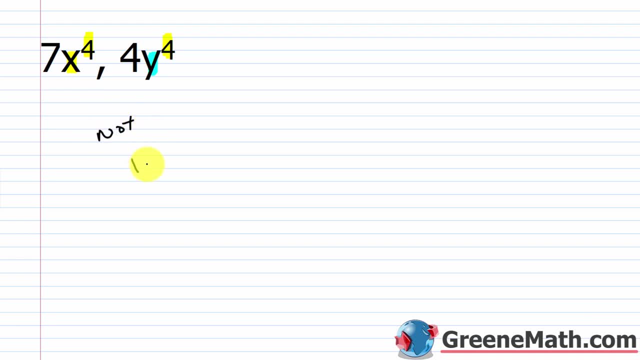 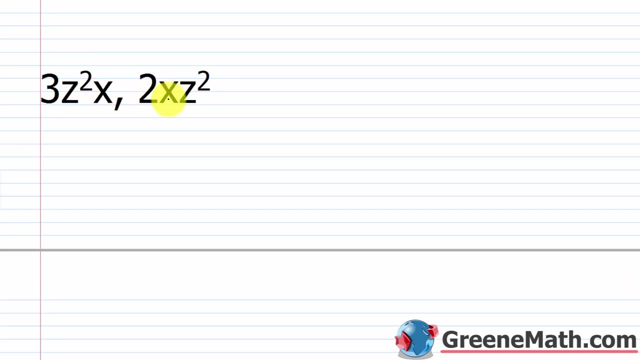 they're different and so they're not like terms. Here we have 3z squared x, and then 2x- z squared, So this one might look like they're not like terms, but in fact they are. The variables are presented in a different order, but I want you to remember. 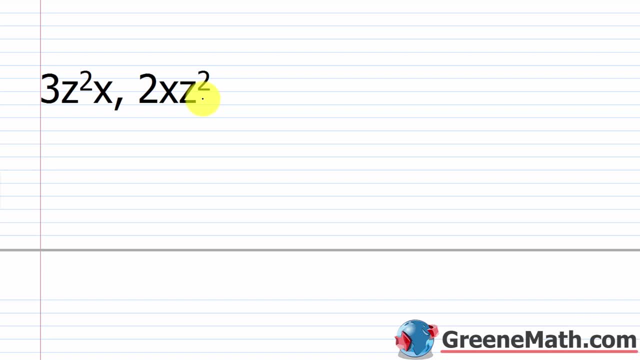 back from pre-algebra that multiplication can occur in any order, right? That's called the commutative property of multiplication. So if I have x, y and z squared, I'm going to have x squared, So I'm going to have x squared. 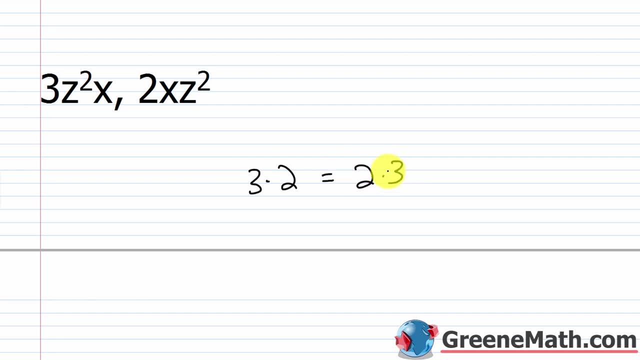 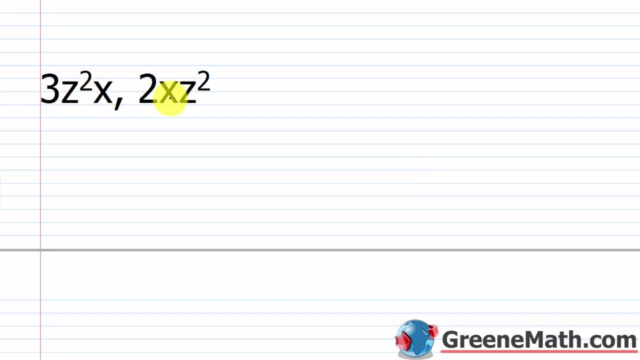 variables in any order. I can have z squared times x or x times z squared, it doesn't matter, right? So I have the exact same variables here raised to the same power. I have z squared and z squared, So put a check mark there, And then I have x and x. Put a check mark there And again. 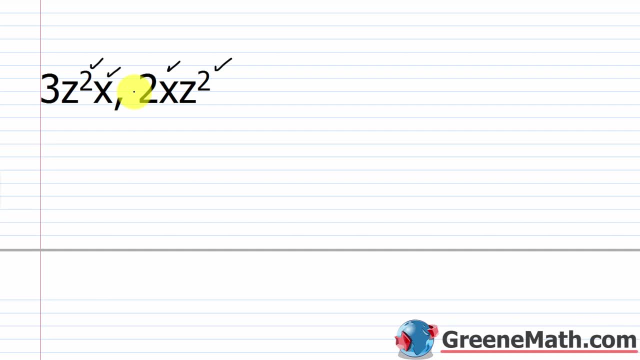 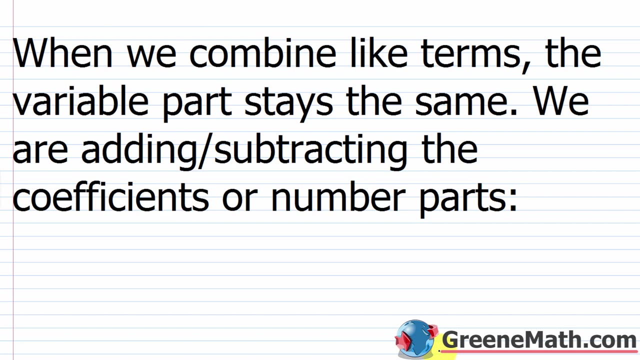 the coefficients can be different. So, because everything is the same, we have like terms, Like terms. Okay, So let's talk a little bit about what we're going to do with these like terms. All right, So when we combine like terms, the variable part stays the same. So, if I have x, 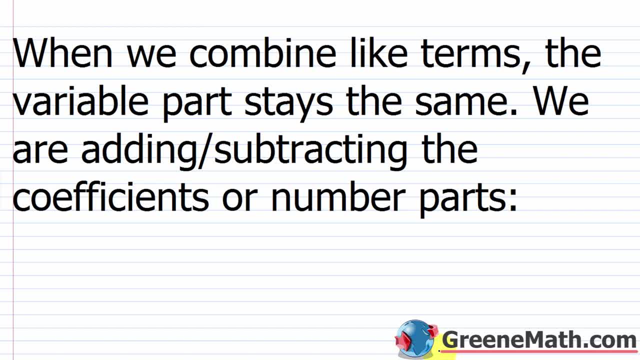 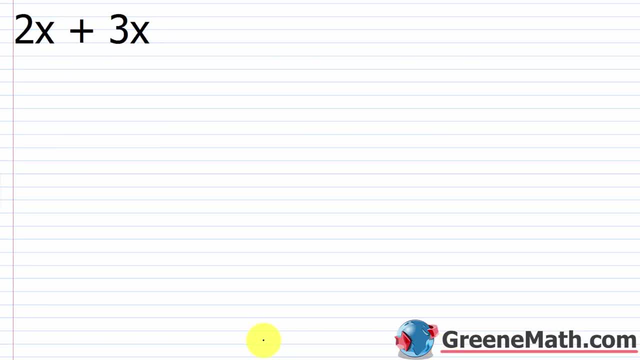 squared and x squared. that doesn't change. We're just going to be adding and subtracting the coefficients, or again, the number parts. All right, So let's take a look at 2x plus 3x. Nice and easy problem. I want you to imagine if you had two oranges. 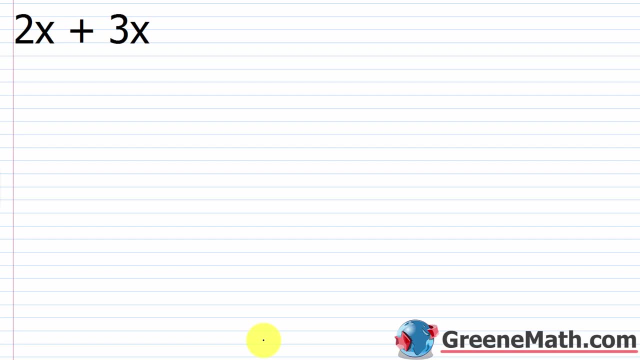 and you added to that three oranges, or everybody knows they'd have five oranges. The easy way to do it is just to leave the variable the same, Just say okay, I know I'm going to have x, And just add the coefficients. So 2 plus 3 is 5.. That's 5x If you were to. 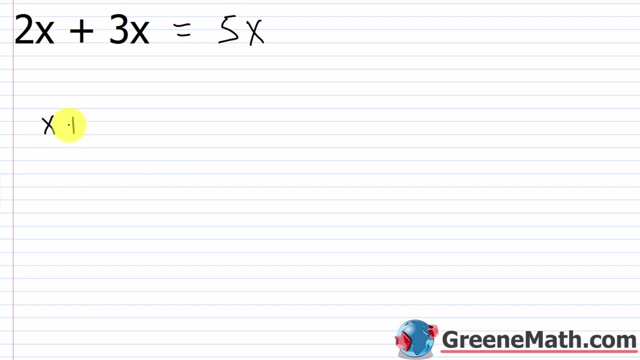 visualize what's going on: 2x is x plus x, So x plus x, And then 3x is x plus x plus x, And if you kind of view it this way, it makes sense. Okay, I have 1,, 2,, 3,, 4, 5 of these guys. 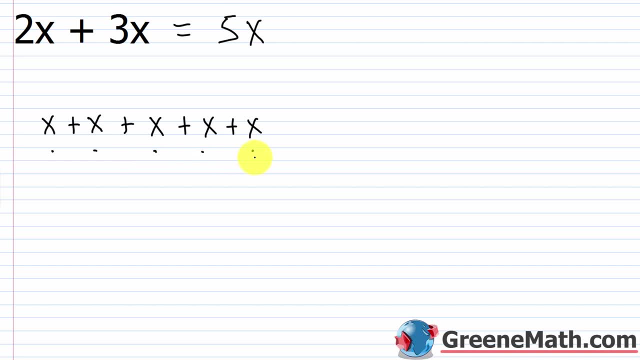 5x. But you don't want to do that every time. It's going to slow you down, Right? So you just want to say: okay, the variable part is going to stay the same, So that x is going to stay the. 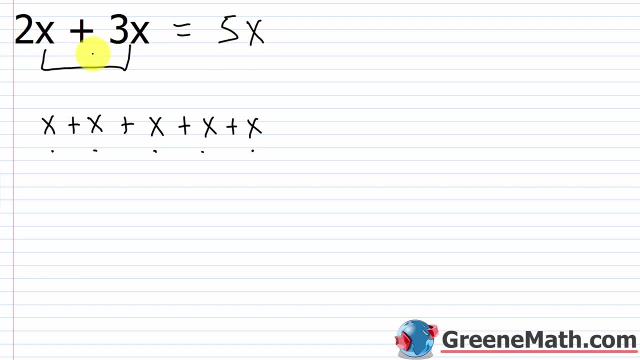 same. So I just write that first, Then I'm just going to add the coefficient parts, Right? So 2 plus 3 is what That's 5.. So I end up with 5x, And again, if I have 2 of something plus 3 of the 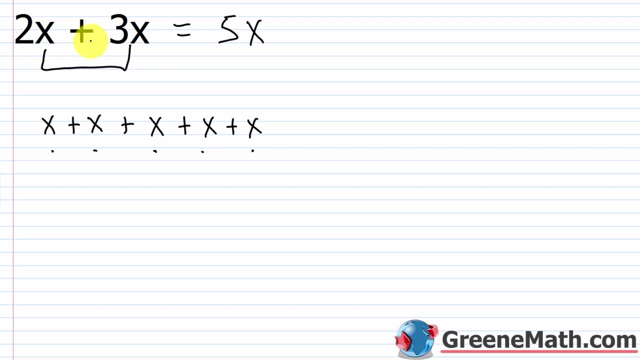 same thing. I'm going to have 5 of something. So 2 apples plus 3 apples gives me 5 apples. 2 Honda Civics plus 3 Honda Civics gives me 5. Honda Civics Right, So on and so forth. Another way to kind of think about it. 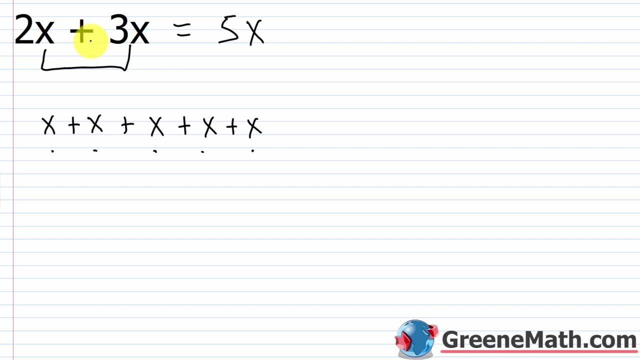 using the distributive property and it involves factoring, which we haven't gotten to yet. But if I were to write this for you like this, let's say that I pulled the x out, which is common to both, And I wrote this as x times the quantity 2 plus 3.. Well, I could do 2 plus 3 first and get. 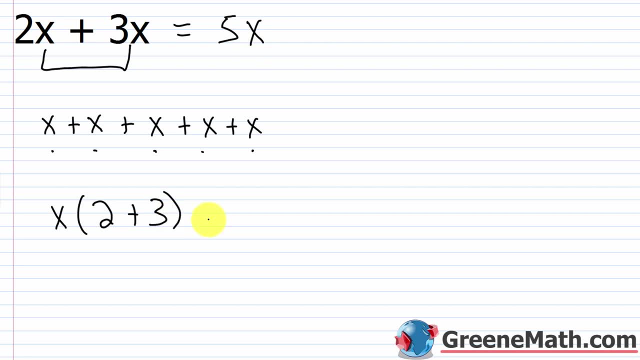 5. Multiply 5 times x. I ended up with 5x. Or I could again distribute: the x x times 2 is 2.. x plus x times 3, which is 3x, And again you see where we start with this: 2x plus 3x. 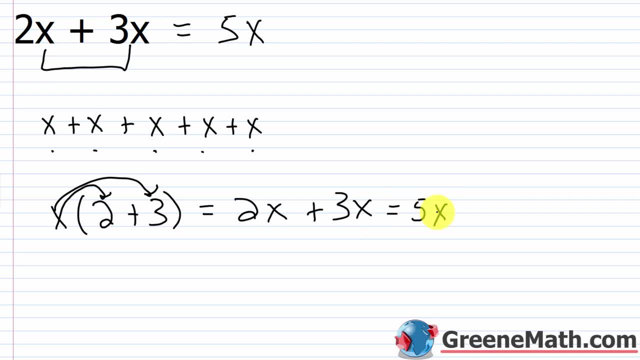 So kind of any way you want to use to visualize what's going on here, it's 2 of something plus 3 of the same thing, is giving you 5 of that thing: 2 apples plus 3 apples, 5 apples, 2 oranges plus. 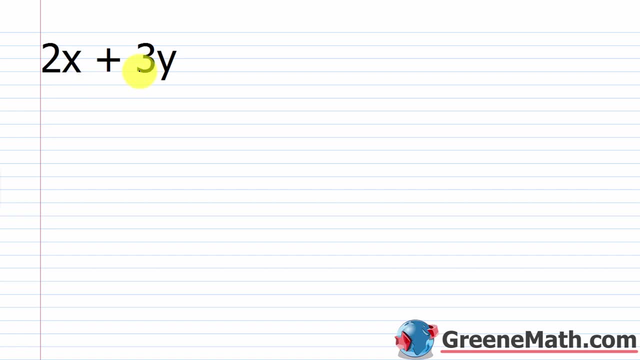 3 oranges, 5 oranges, So on and so forth. Here we have 2x plus 3y. Now we don't have like terms here, So we can't get 2x plus 3y. So we can't get 2y. So we can't get 2y, So we can't get 2x plus 3y. 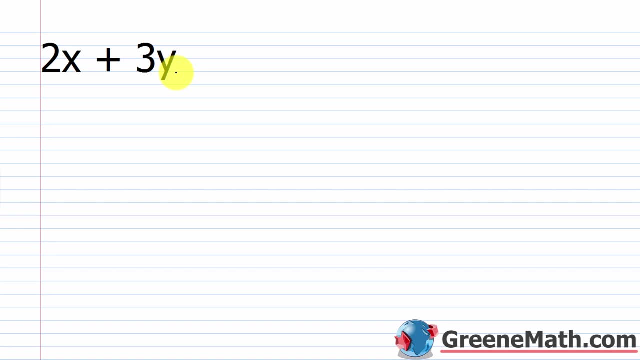 can't combine them. So let me try to make sense of this for you. If I have two, let's say- oranges and I try to add that to three apples, well, I still have two oranges and three apples, right? 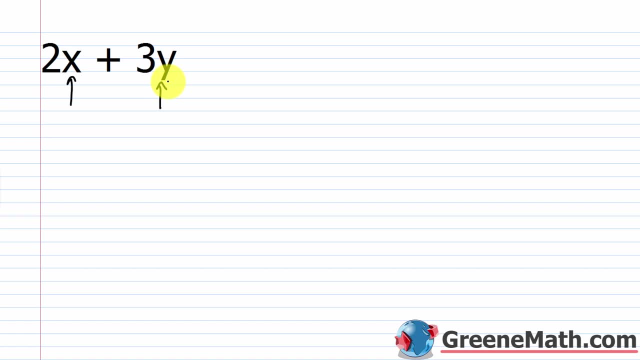 I can't combine them and say, okay, well, I have five orange apples, right? I don't? In the case where we had the same variable, right, we had like terms, well, yeah, I'm adding the same thing. So if I have again two oranges plus three oranges, I have five oranges If I have two apples. 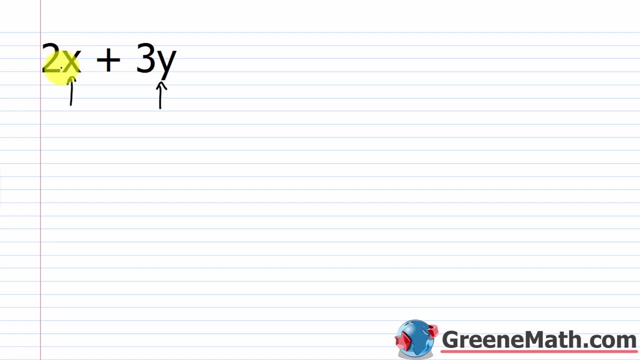 plus three apples, I have five apples. But if I have two oranges plus three apples, I just have two oranges and three apples. So there's no way to, kind of you know, combine these. It's still going to just be 2x plus 3y. So if you don't have like terms you really can't simplify. 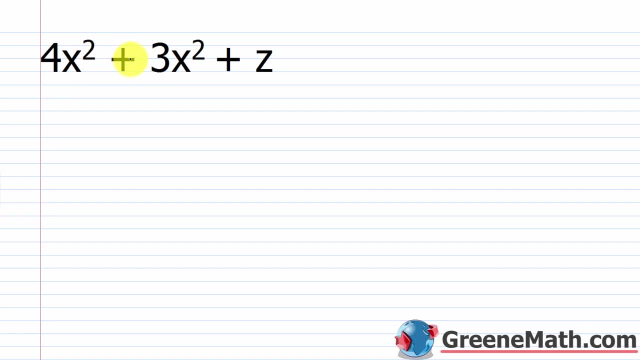 right in this scenario. All right, here we have 4x squared plus 3x squared plus z. Now look for your like terms. I have x squared and x squared, So these two are like terms. These are like terms And so we can combine them, And I missed. 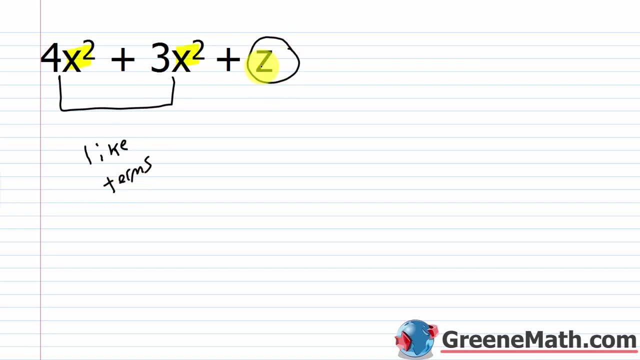 an r there. The z is not common to anything, right? So we're not going to have like terms with just the z. So what you do in this scenario is you just combine what you can. So 4x squared plus 3x squared Again, leave the variable part the same. So leave that x squared part the same. 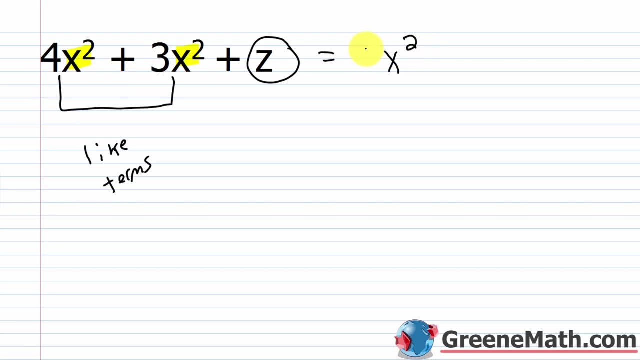 And then just add your coefficients. So what is 4 plus 3?? That's 7.. So I have 7x squared And then just copy the rest, So plus z. So when we simplify this algebraic expression, we end up with 7x squared plus z, right Again. 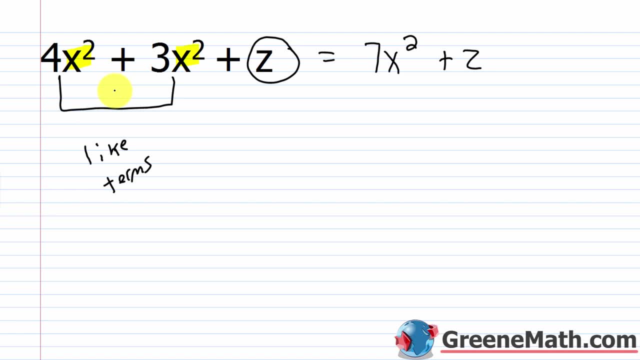 you combine what you can right. In this case, we could combine the like terms 4x squared and 3x squared. All right, here's one that's a little bit more challenging. We have negative 2 times the quantity 4x minus 7, plus 4 times the quantity x minus 3..